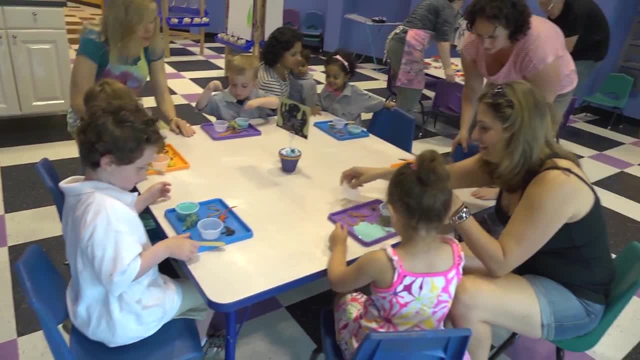 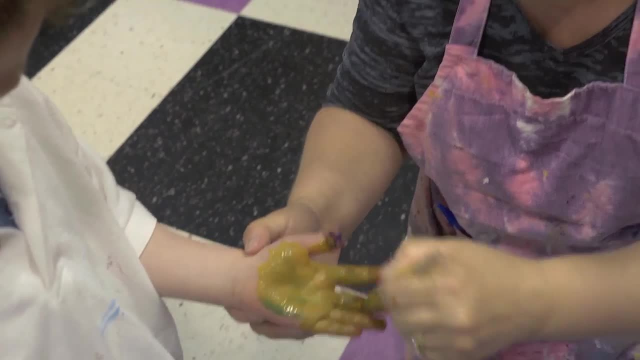 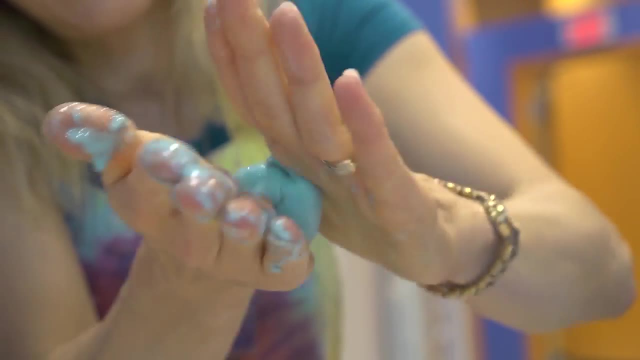 I'll hear parents tell their children: wait. you have to wait for the teachers to tell you what to do, But the children come running in and they know what to do. They don't need instructions, They'll dive right in. It's like a solid when we roll it in a ball. 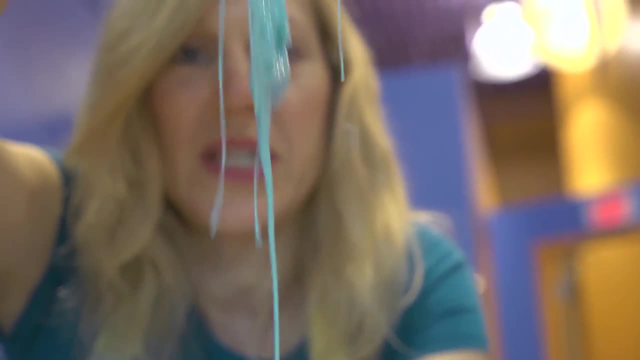 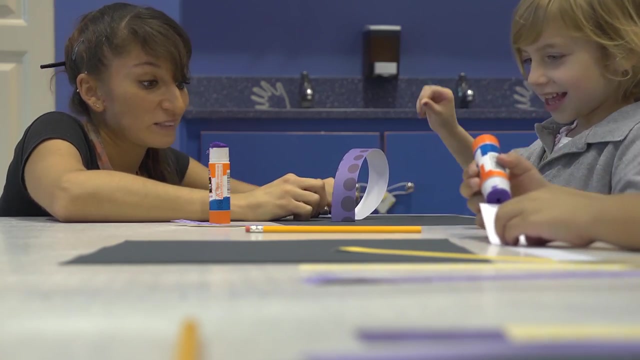 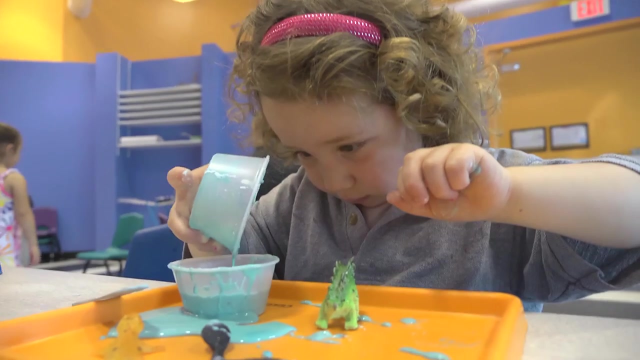 And then, when we stop, it just oozes into liquid. Our teachers have found a way to teach art to children that helps them express their emotions And find themselves, And to explore art in so many different ways. It's not all about the art. 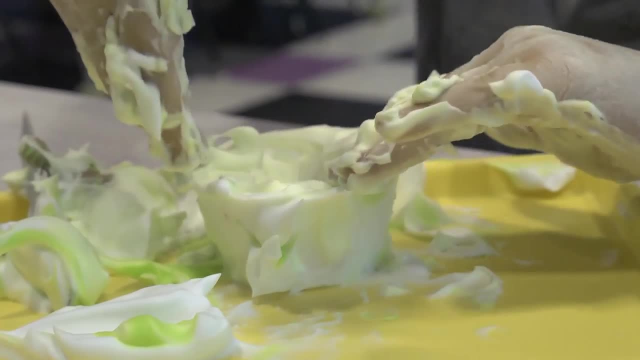 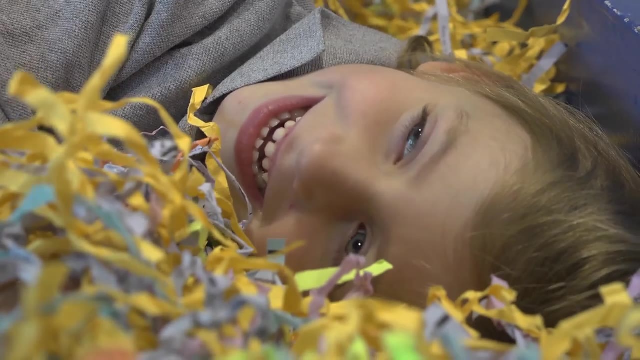 It's about exploring and playing and learning through your senses. Playing with shaving cream, slime and goop, Exploring different textures and materials. Our sensory box is the highlight. for every two-year-old. We have about five different sand boxes, although we never do sand. 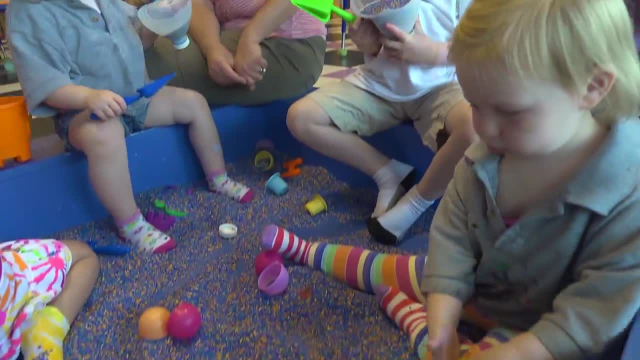 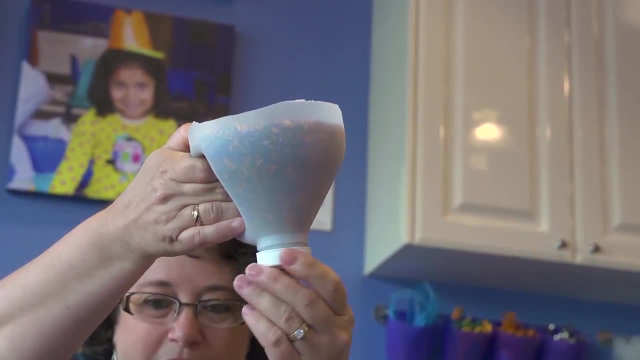 We do colored rice, shredded paper, squishy balls. My favorite are the recycled gallons of paint bottles. The children scoop up the rice, unscrew the cover and the rice comes pouring through One, two, three. It's visually, auditorily and intellectually stimulating. 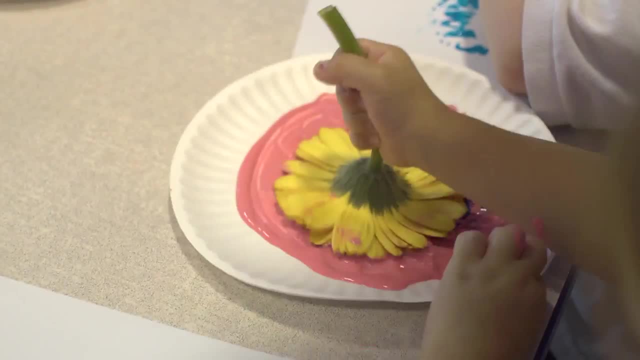 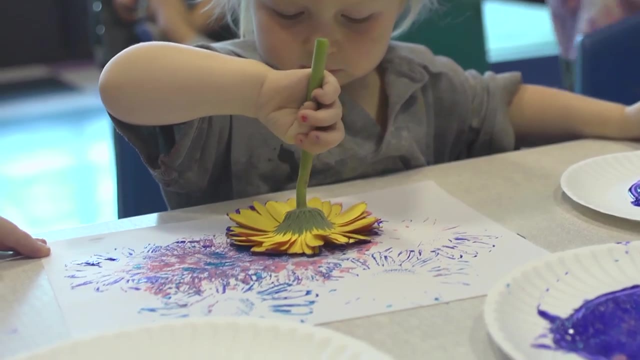 We love to use a variety of tools and materials in new and novel ways. Painting with flowers is one of my favorite activities. We use great big Gerber daisies, dip it in the paint and make prints. It's gorgeous every time. 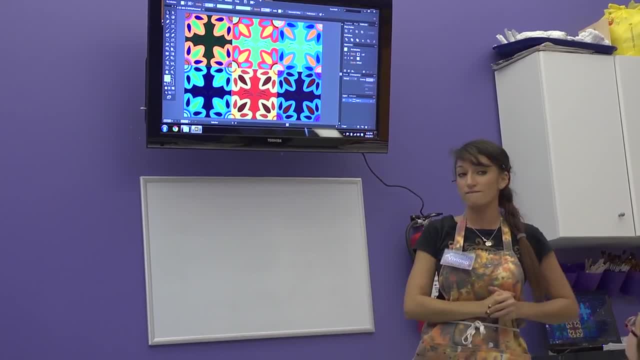 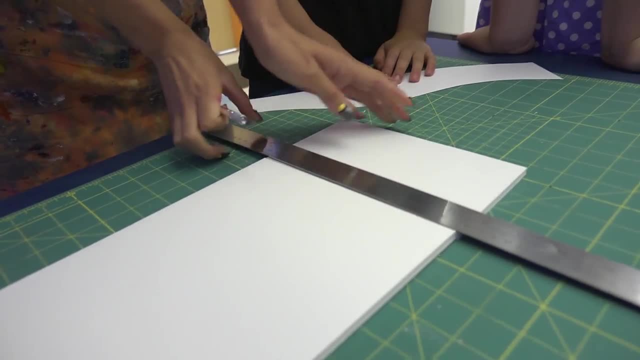 Can you guys find the one that's primary? Do you know which one it is? As children get older, we begin to add more structure. The teacher does a short lesson and then they do their project. The lesson may be learning about patterns or symmetry, complementary colors. 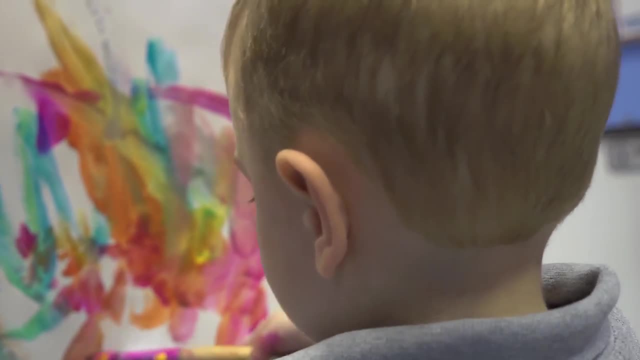 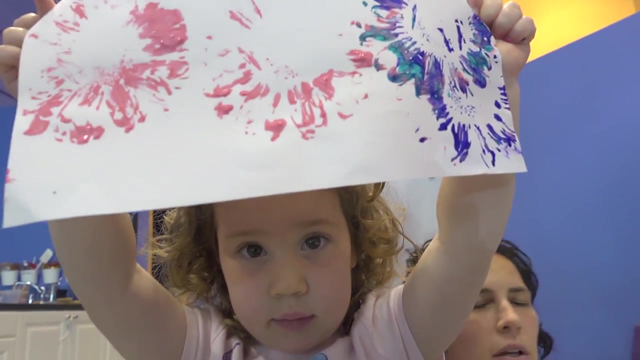 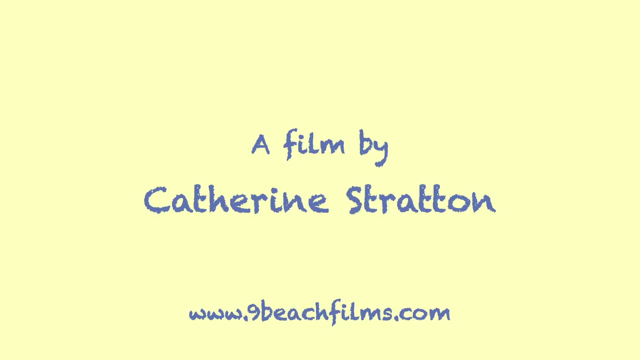 I love when I see children creating in a new and innovative way that we never even thought of At the Messy Artist. art could be a masterpiece of whatever they want it to be. I hope you'll join us next time, Thank you. 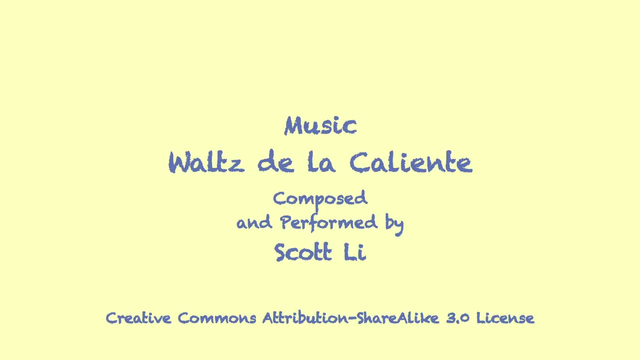